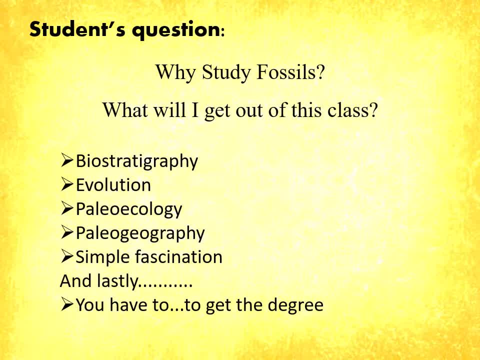 vague term and that is mislead us. Basically, it's the remnants of the ancient organisms which live in that time. they are preserved in the rock record which we called as fossils. Basically, the study of fossils, that is, the ancient organisms, is known as paleontology. 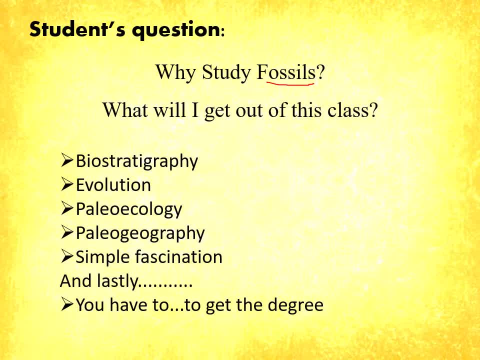 Now a student may ask you that: why should we study paleontology or why should we study fossils? What will I get from this class? What scientific information it will provide us to understand the history of the earth. The first and foremost information, scientific reasons or scientific. 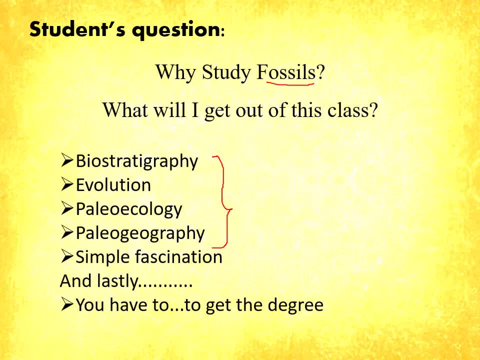 informations, what you get by studying paleontology. Apart from this, there are several minor informations are also get when you study the subject paleontology. The fifth thing is people's study paleontology due to simple fascination, because you are also studying the biological part in your subconscious mind, because whenever you go into some beach areas in the near conditions, 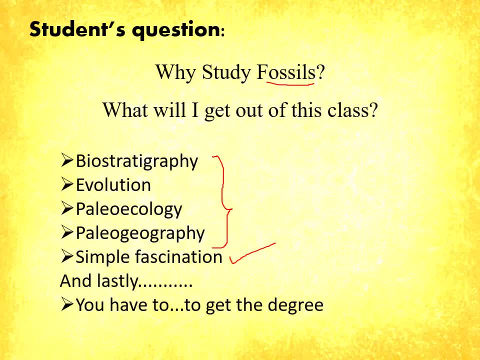 of any sea, you will find different shells of bivalves and gastropods, that is, different types of cells, different color of cells of your shamook and chirnook. So, whether you know about their biology or whether you know about their ecological conditions, whether 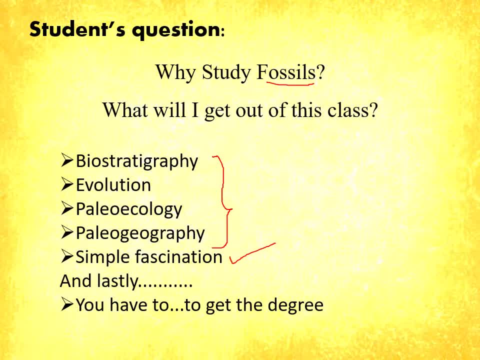 you know about their habitat. Most of us, we all, did not know about these things, about the biological aspect of those cells. But instead of that, we are collecting those cells. Why we collect? We did not know anything about those organisms, about those cells. 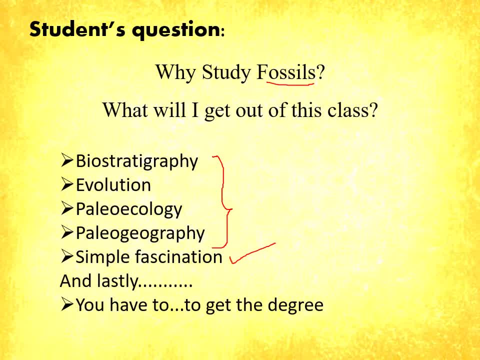 But still we collect, sometimes we buy from the nearby shops. That is because they are very attractive and because of their attractiveness We sometimes collect them. We sometimes study the minute things or the broad things, such as their shape, such as their color. Those things are studied and noted. 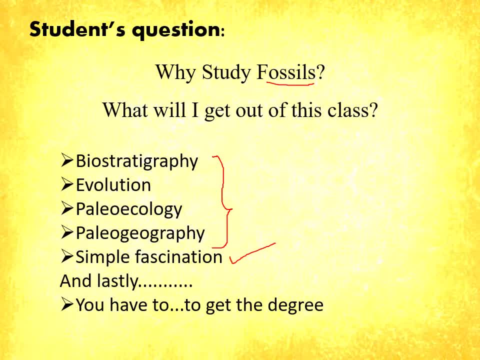 So, simply due to fascination- people love to do that- They will also study the subject paleontology. And lastly, that is proposed by me for the students: You have to study paleontology, whether you like it or dislike it, to get your graduation degree. 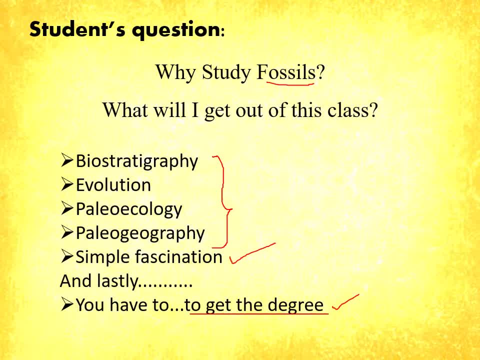 Because there is a subject called paleontology in your syllabus And it have a pretty much mass contribution in your total number of your undergrad study, And if you are not able to pass this subject then you will not get the degree. So whether you like it or not, you have to study. 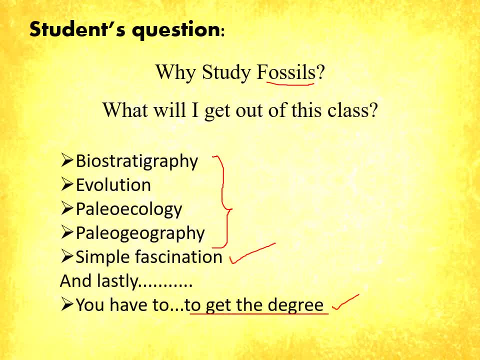 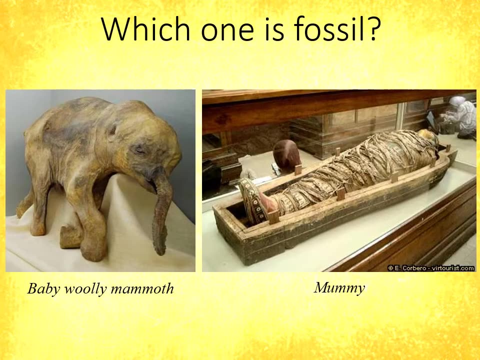 But this subject is very much interesting If you try to understand the basic things, the basic phenomenon behind it. Now, here I am, showing you two pictures. The first one is a baby woolly mammoth And the second one is a mummy. 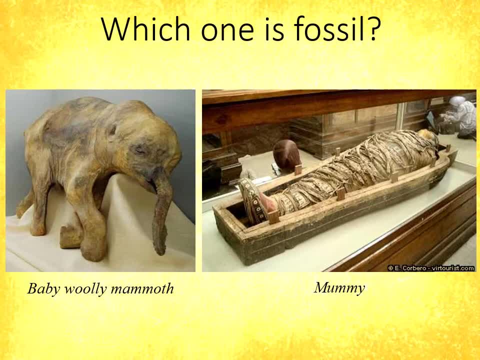 Now can you say which one of these two Is fossils, whether it is a baby mammoth or a mummy, Because we all know that all these things are not present during this time. A baby mammoth present in the earth about 20,000 years ago. 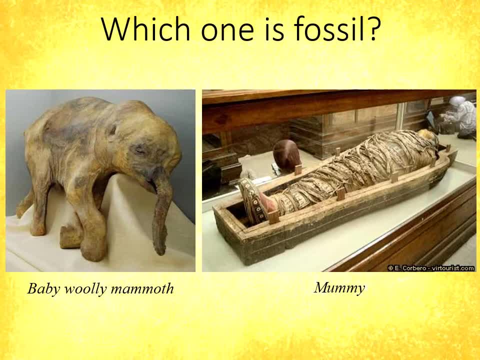 Whether is a mummy is a human, But these humans present far ago from the present day times And they are mummified after their death. So this dead body present within this coatings, They are not of present day time, So that is why I called it. these are ancient human bodies. 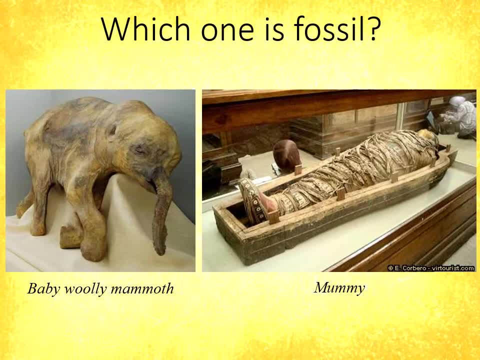 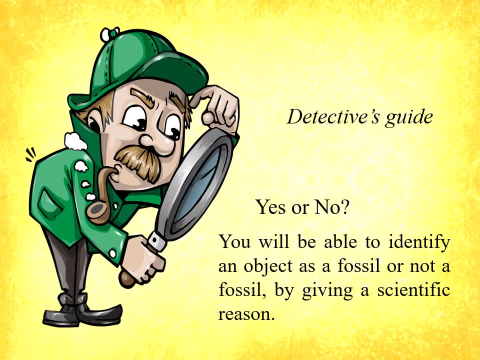 So which one is fossil, a mammoth or a mummy? Now you have to answer this question. So whenever you try to answer this question to your closed ones, If someone asks you: okay, you are studying paleontology, So tell me whether a mammoth, between a mammoth and a mummy, which one is fossils? 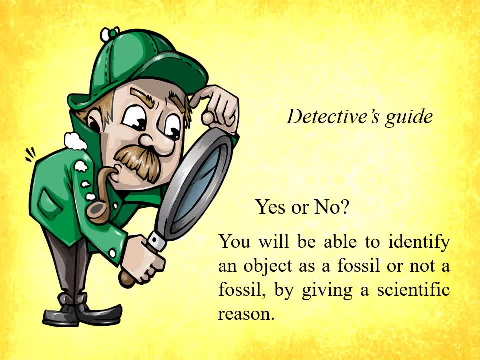 So you have to think from the scientific point of view. You cannot answer randomly, But you have to think from a scientific point of view And justify to your answer by some logical approach. So you have to be a detective to find out the clue to say any particular thing. 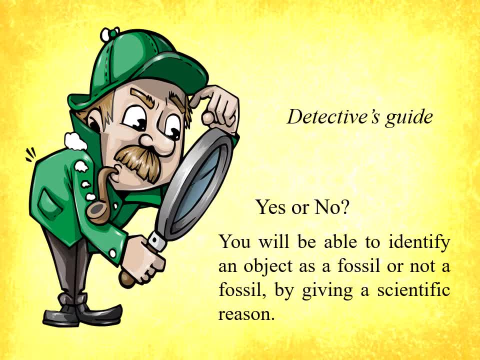 That is to say, whether the mummy is a fossil Or whether the woolly mammoth is a fossil. So before giving answer to anybody, You have to identify the clue And you have to give them a scientific reason Due to which you called someone. 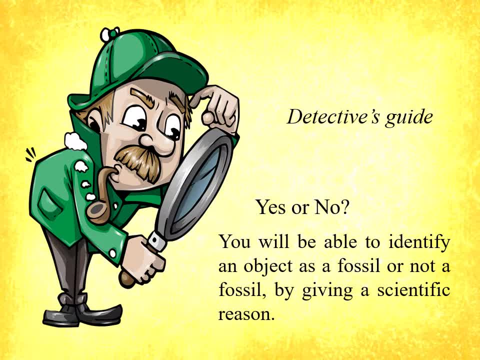 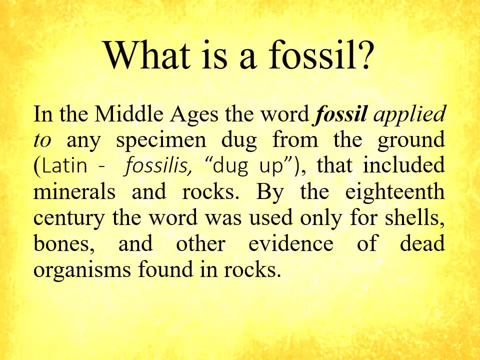 A fossil. So basically you have to follow a detective's guide. Now, what is a fossil? So in its earlier times, That is, in the middle ages, Basically the word fossil applied to any specimen. Basically it comes from a German word Which means exceptional preservation. 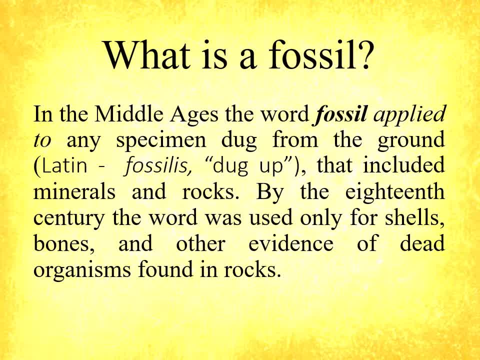 Or exceptionally found. Now, in the middle ages, The term fossil is applied to any specimen Which is dug from the ground surface. So it may be an ancient living being, Or it may be a mineral, Or it may be sometimes people dug for water. 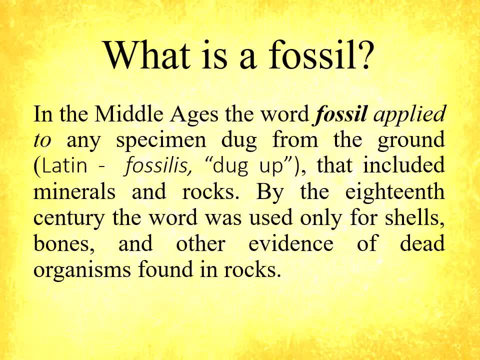 To establish any fuel. So the question comes: If we dug for water And established a fuel, Then can we call water as fossil? Because in those times Anything which is dug up- That include minerals, Rocks, Ancient organisms- Are called fossils. 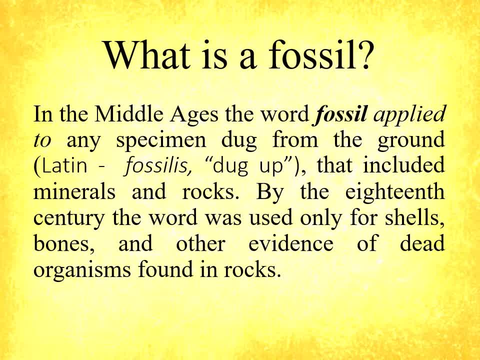 So people Are mislead By the term That. whom should we call fossils Or whom we do not call fossil? By the 18th century The word gets its Precise meaning, That is, We called fossils Only to those things. 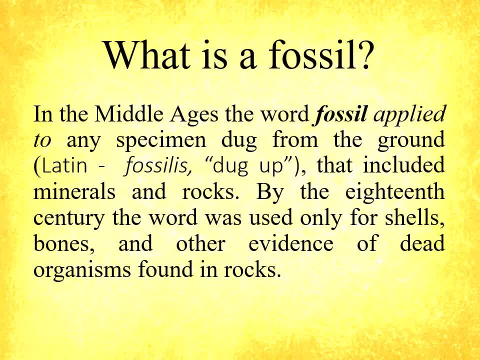 Which belongs to Some ancient living entities Preserved in the rock. So you can see That whenever We called For, the term fossil Is only applicable to the Ancient living beings, That is, their shells Or any part of their 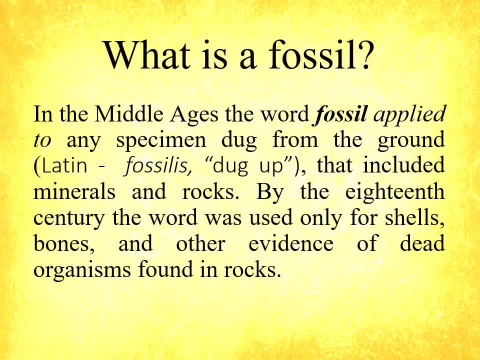 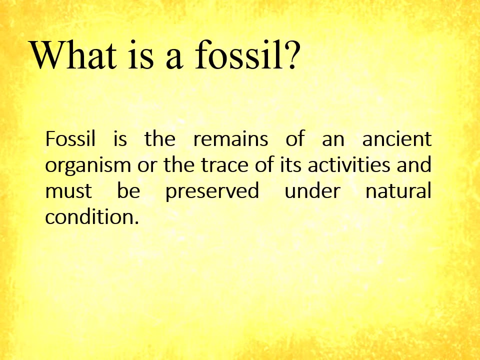 Body, Then Automatically We are discarding these things. So only the ancient Living beings Or their Remnants Or their traces Are called fossils. Now If we try to define the term Fossil In proper scientific 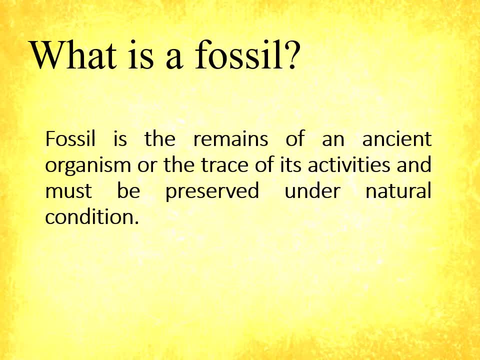 Language, Then Fossils Are the remains Of ancient organisms. It may be the complete organisms Or it may be part of the organisms, But It will be the Remnants of ancient organisms Or The traces Of it activities. 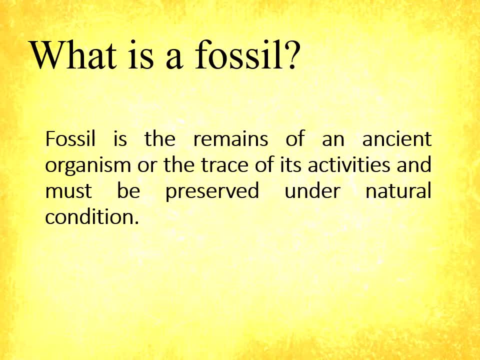 Must be preserved under Natural conditions. So Three things You will get from these Definition. First, It must be Remnants Of ancient organisms. That may be the complete Remnant, Complete Organisms Preserved. 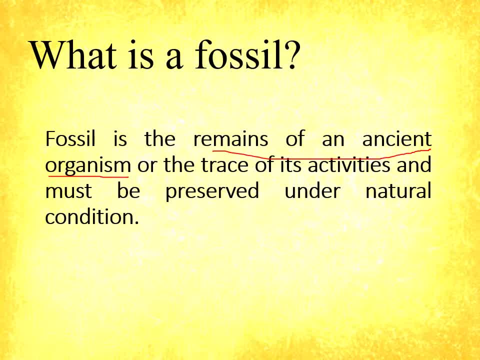 Or part of the organism Preserves. Both are called fossils. Or sometimes The organism Is not At all Preserved, But It's Activity Is preserved In the natural Condition. So It's Preserved. 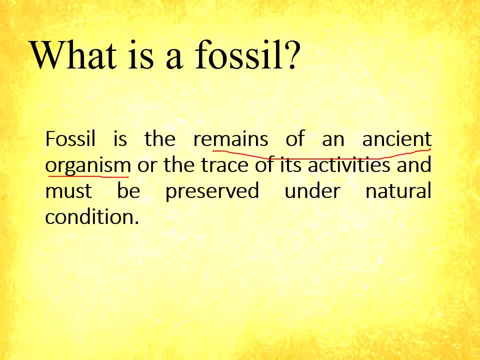 In the rock Suppose You are running Over A sandy surface And Your footprints Are Following You. So You are moving In the forward Direction, But Your footprints Stays Behind. 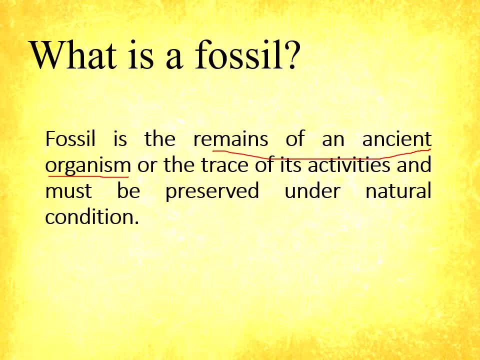 You. So If someone Want To study Your footprints Then They can Say: Sandy Surface Just By Studying Your Footprints. So Those Footprints Are Basically Indicate. 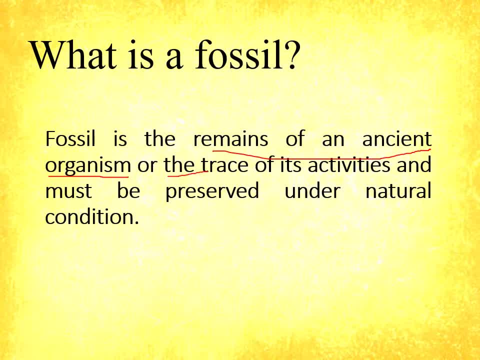 A Activity Done By You. So In Those Cases, Those Activities, Those Traces Which Are Indicative Of Your Footprints. So, If You Want To, 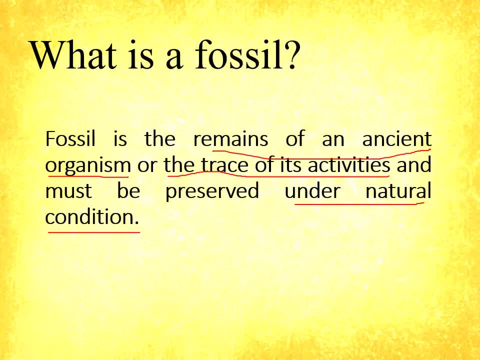 Study Your Footprints, Then Your Footprints Are Indicative Of Your Activity. So If You Want To Study Your Footprints, Then You Can Use. 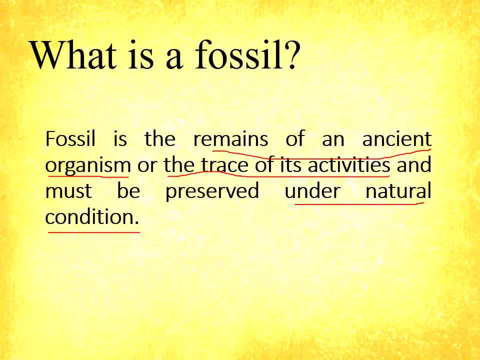 Your Footprints To Find Your Footprints. So If You Want To Study Your Footprints, Then You Can Use Your Footprints, Then You Can Use. 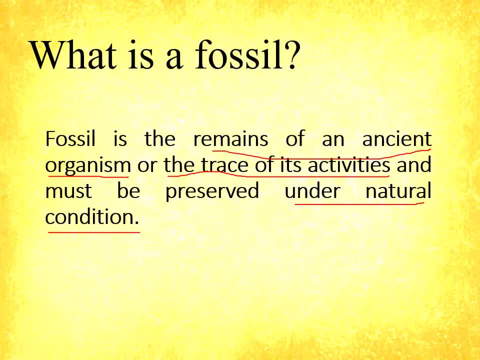 Your Footprints To Find Your Activity, Your Activity. If You Want To Study Your Footprints, Then You Can Use Your Footprints To Find Your. 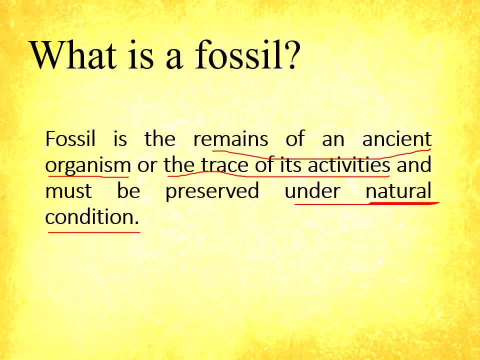 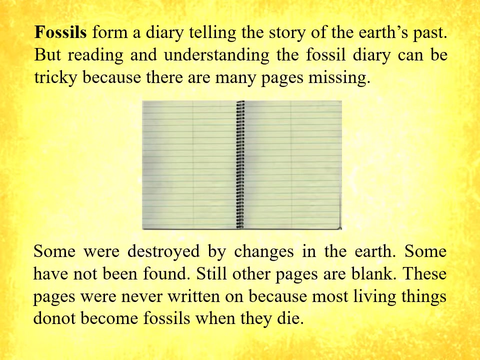 Activity, Then You Can Use Your Footprints To Find a fossil. you must be very much aware that that is preserved under natural condition. now, fossils is basically reading a story from a ancient diary. there are many things written on the diary in page wise, so you have to. 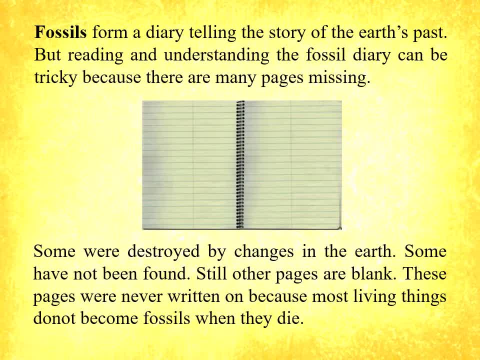 understand that writing and you have to study those writings very carefully. but it often happened that in an ancient diary many pages are torn up or many pages are actually missing. in natural world that is also happened. we all know from our previous classes that anything which is deposited in any time, 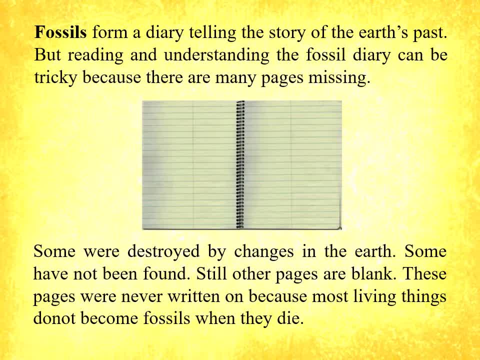 their preservation is very rare, but being not preserved is the most common thing. so anything living being present at any particular time interval, whether they will preserve, and going to the fossil record or not, that is simply a chance factor. so it may often happen that many fossil evidences 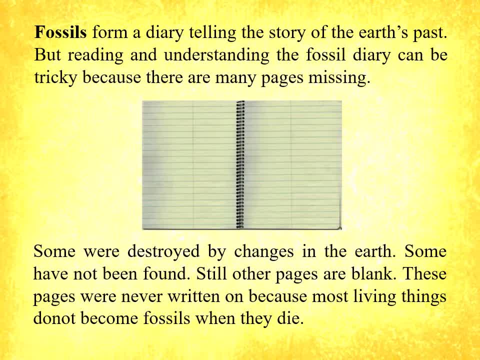 many organism evidences of ancient life. they are destroyed in due courses through time. so whenever you try to study the fossil diary, try to study the fossil evidences from the sedimentary rock record, that is, try to study the organisms through time. you must be very much careful. 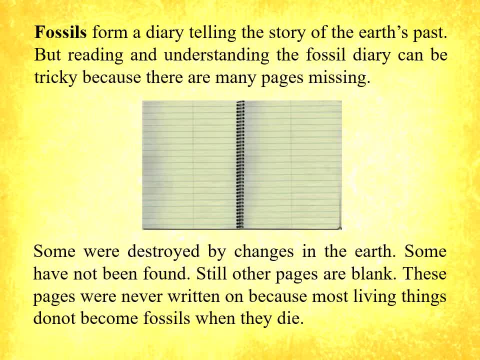 whether all the pages of the diaries are there or whether there are any biological evidence in the fossil record. and also what are the characteristics of the fossil records. that means whether they are a continuous sequences of fossil evidences or some. there are some missing things in the fossil in most cases, or it is very common. 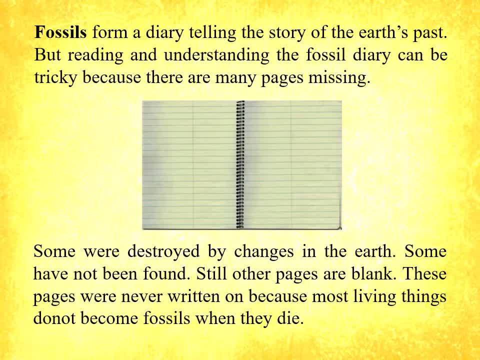 that the fossil record is incomplete, that is, most of the organic evidences are not preserved in the rock record, but still it's very interesting to someone, for someone who love the organic world, because it tells us many things, many, many informations, about the ancient organic world, as well as it tells us how. 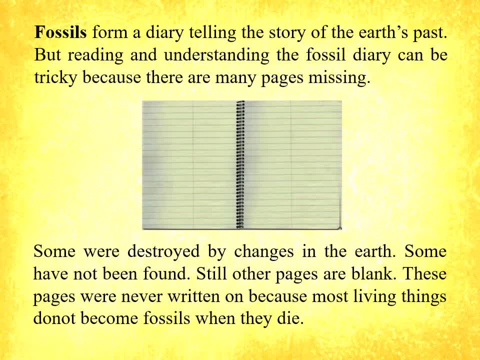 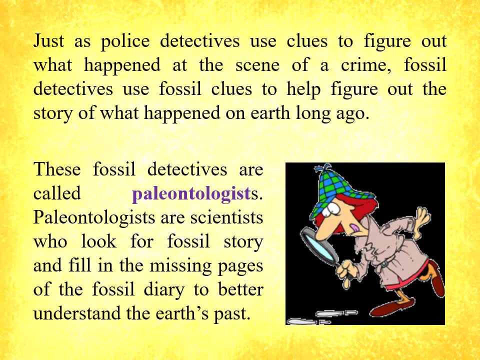 we came and how long will we sustain in the present day earth? so, just as a police detective, you have to use the clues, what happened at the crime scene, that means what happened during the deposition of the sedimentary rock, and you have to figure out the story behind those organic bodies, ancient organic bodies. so those peoples? 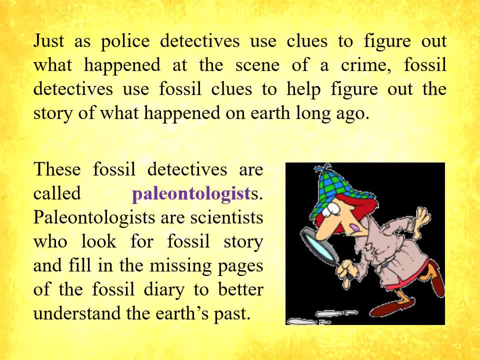 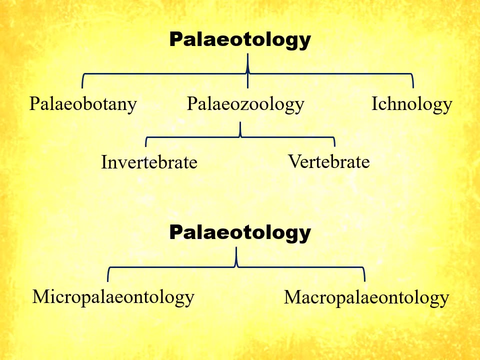 who study these ancient organisms are known as paleontologists, so the subject is paleontology, and those people who study paleontology or who do research, who do research in the subject paleontology, is known as paleontologists. now paleontology can be branched into several sub branches where the 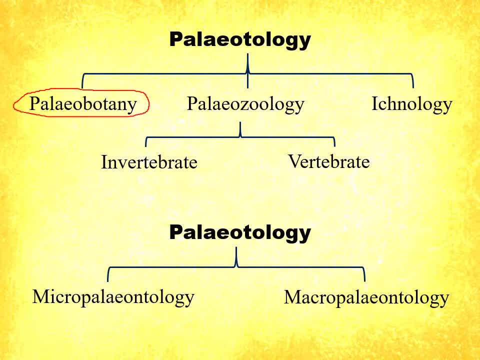 ancient plants are studied, that is known as paleobotany. when ancient organisms are studied, it is known as paleontology. and when the plants are studied and spread around, plants, even in nature, live life, but paleontology cannot be studied when there are only some Yesterday high princes or your ancestors, smells of rges and there is a way that they Fight Quality Unfairness. 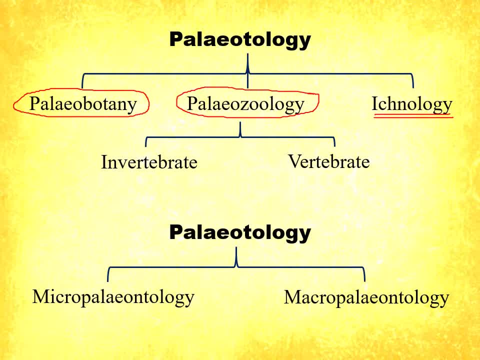 of traces of organisms. now paleozoology can again be divided into two branches. one is the invertebrate paleozoology, another is the vertebrate paleozoology, depending on whether the organism, whether the animal body, have vertebral column or not. so this is the broad divisions of paleontology. 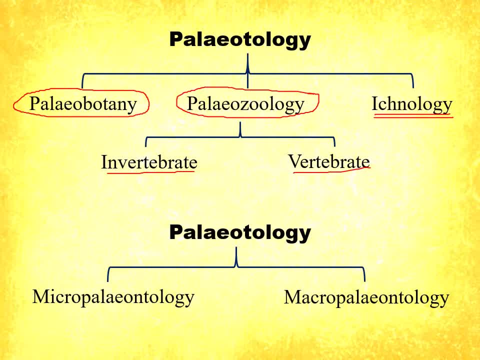 now paleontology can be again subdivided into two halves. whether they are studied under naked eye, that is, in simply naked eye, or with the help of pocket lens, or the evidences of organisms or the details of organisms are studied under the common petrological microscope. so when they are studied, 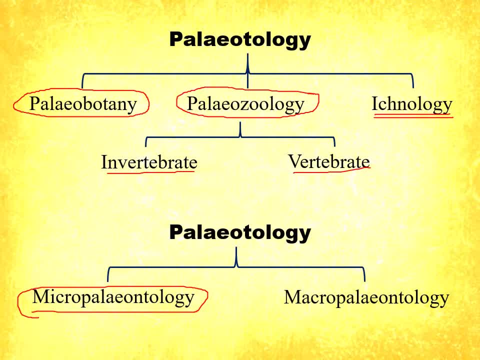 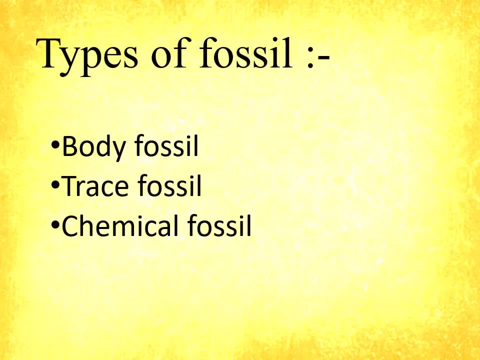 under microscope, they are known as micro paleontology. when they are simply studied under naked eye, they are known as macro paleontology. now, what are the types of fossils which we are studying during a study of paleontology? so three types of fossils are classified. the first one is the body fossil, when the entire 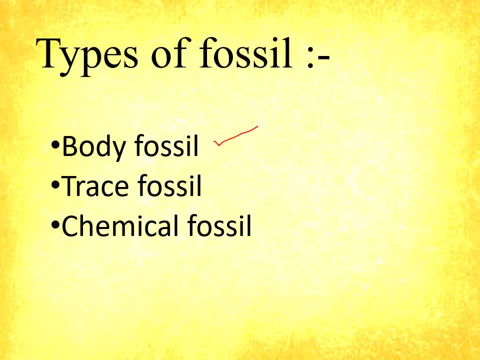 or part of the original body of the organism is preserved and that body means and that if you may very well aware that, simply, if you consider the body of human being, and the human body is- consists of several hard parts, those are the bones, cartilages, and several soft parts, several muscles. so any 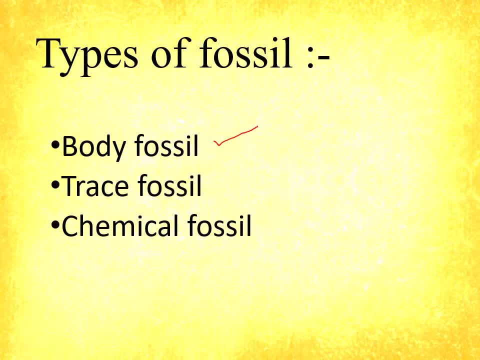 of an organism and in most cases the body of an organism consists of two parts: the hard parts and the soft parts. in body fossil they both may be preserved, that is, the hard parts and soft parts. both may be preserved, or only the hard part or only the soft part can be preserved. but it is found 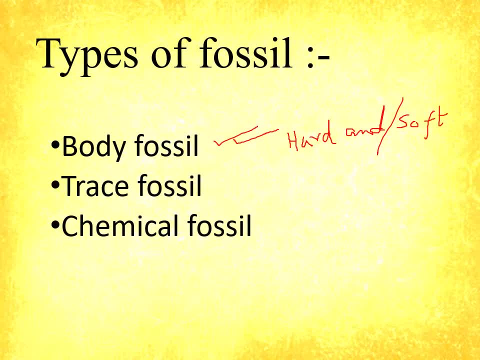 that whenever an organism died, the first thing is that the soft part of the organism, that is, the muscles, tissues, they are decomposed. you may often find a dead body of an animal, dead body of a dog or dead body of a goat in the roadside. so you will find that after some days it will smell terrible, and this smell is 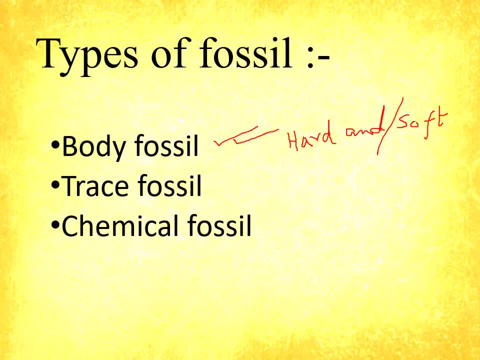 because, due to the decomposition of the muscles of the dead body by some decomposing bacteria, but when the decomposition of the soft masses, when the decomposition of the muscles is complete, still the hard parts, the bones, remain as it is. so generally, hard parts have more tendencies to be preserved, more chances to be preserved, compared to the soft parts, compared to the muscles. 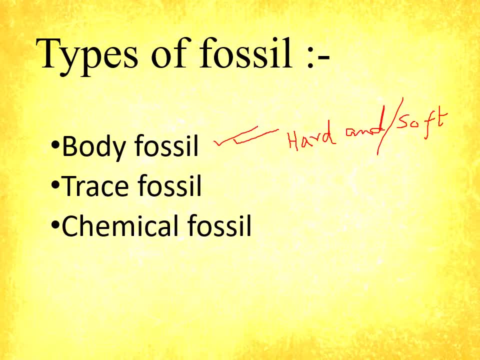 so when you consider a body, fossil, that consists in the entire body or part of the body, or it consists only the hard part of the organisms, or it consists the hard part and soft parts of the organisms. so any part of the body or the entire body of the ancient organisms, if it is preserved. 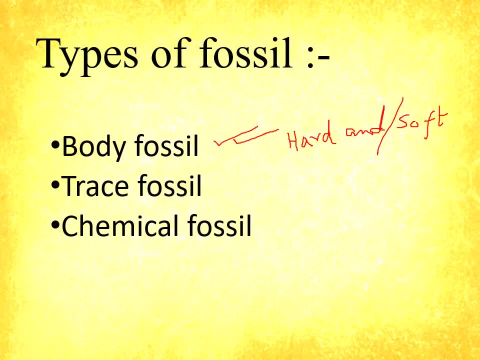 naturally, then we call them as body fossils. mind it, whenever you have to define body fossil, you have to mention that it is preserved naturally. that is the first and foremost criteria to call it a fossil. second is the trace fossil. as i already told you, in trace fossil you are not getting the direct evidence. 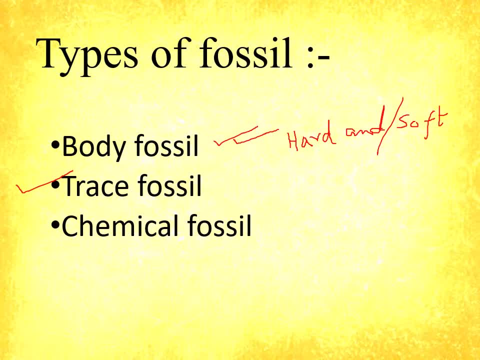 of the body parts of any organisms. instead, you are getting some traces of any kinds of activity of the organisms, say, for example, the footprints of any living being running over any soft sediment, sediment- and after they ran away you can see that they are not getting the direct evidence of the body parts of any organisms. 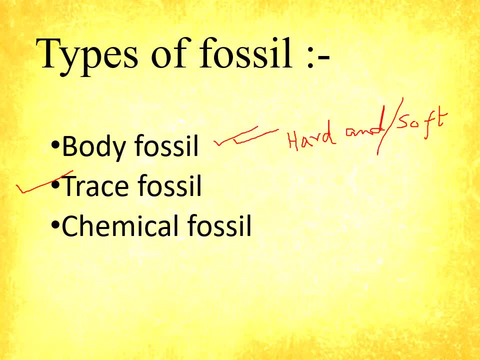 those footprints are preserved in the sediments and in due course, in the latter time, when those footprints are discovered in the rock record, it indicates that certain kind of animals are run away over this sedimentary horizon. so those footprints indicates the running activity of certain kinds of animals and 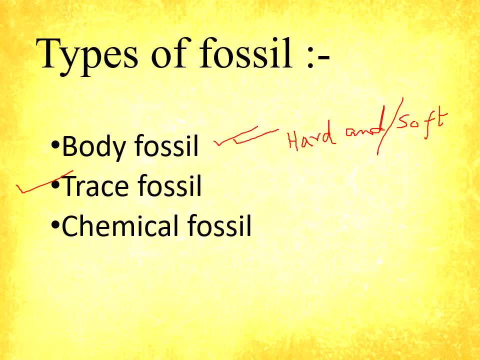 you may know that the fruit prints the periphery of the footprints or certain measurements of the footprints. from though that you can basically estimate the height or the body weight of the organisms, so footprints are also indirect evidences of organisms activity, as well as the shape or the height of the 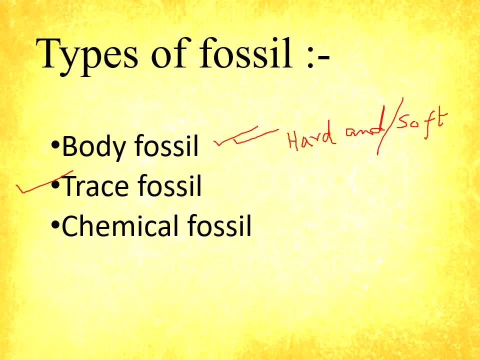 organisms. and the third one is the chemical fossil. it is also an indirect evidence of organic body present in those times, present in the during the deposition of those sediments. basically, instead of getting any body part or getting on traces of activities, here are some chemical components of the organic body mixed with the sediments and whenever we study the 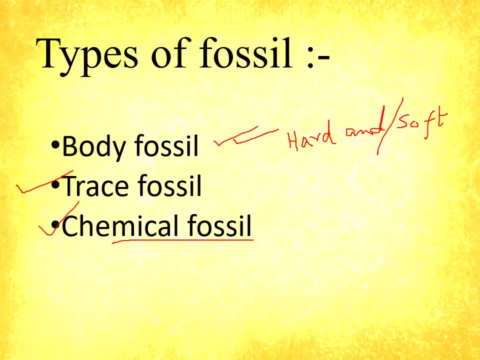 chemical components, that is, whenever we study the chemical analysis of those sediment, sedimentary rocks of that particular point or that particular area, we get some anomalies in this with respect to the surrounding sediments of the same bed, say, for example: uh, you are walking around a road and somehow your finger is cut, so some bloods are. 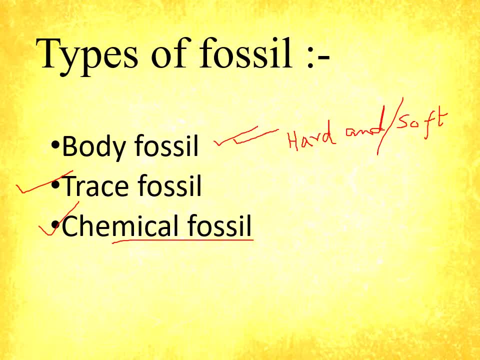 going out from your hand and that blood drops are fallen on the ground surface, so that blood is basically chemical component and it is mixed with the sediments of that particular point. so in that particular point if you do some chemical analysis you get some abnormalities corresponding to the other places where those bird drops are not mixed. 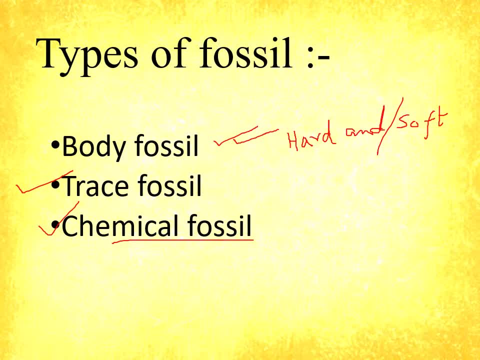 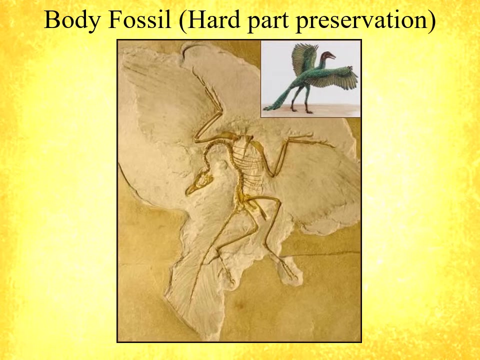 so that is an indirect chemical evidence by which you will get an idea that certain kinds of organic activity is going on over here. so those in those cases they are called as chemical fossils. those chemical traces are known as chemical fossils. here you can see a body, fossil of archaeopteryx. you can see that, all the hard parts, all the bones. 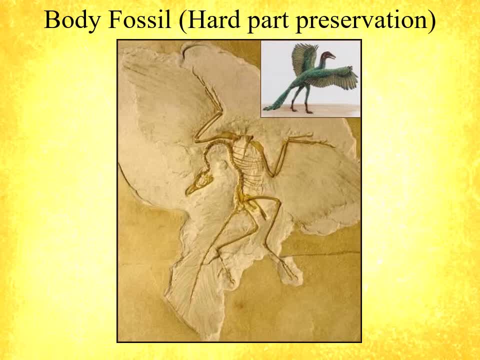 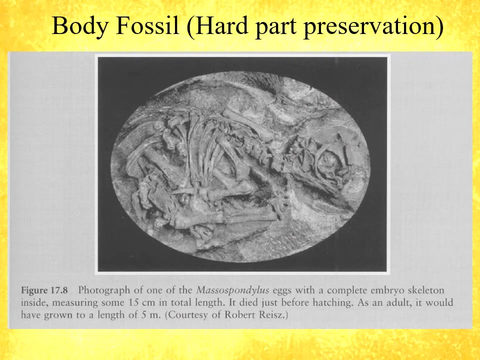 along with the soft parts, that is, the feathers. they are very much, very well preserved. you can very well say: these feathers, these feathers, they are very well preserved. so there is an body fossil almost entirely present. only the soft muscles are not preserved. here again a body fossils, some reptilian egg. this is an egg and within this egg the embryo. 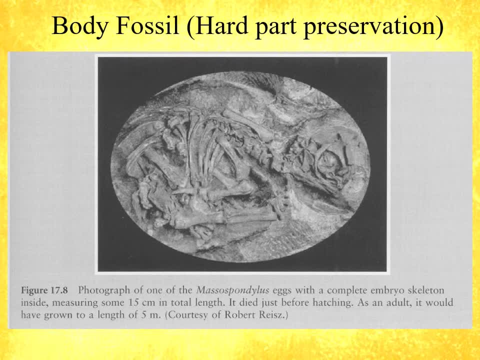 died and the preserved. so it is not um. this egg shape is not formulated, but it is the original egg in which, within this egg, somehow the embryo died and it preserved. so you can see that all the bones are already formed, only thing: the muscles are not preserved. so it is also a 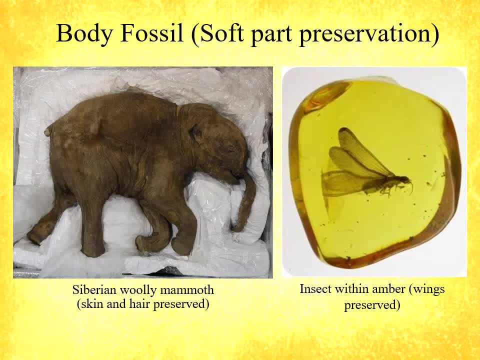 body fossil where the hard parts are preserved, uh body fossils where only the soft part are preserved. this soft part preservation is an unusual thing. in most cases, after the organism dead, the readily decomposed thing is the soft part, that is, the muscles, tissues. they are readily decomposed. 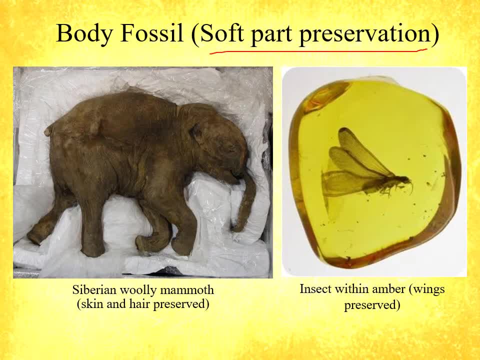 because the decomposing bacteria readily acted over them and they destroy all the soft muscles. so whenever you found a soft part of any organism, that is, the muscles or tissues of any organism, they are very rare and they must be preserved in an unusual case such as this siberian uli mammoth. 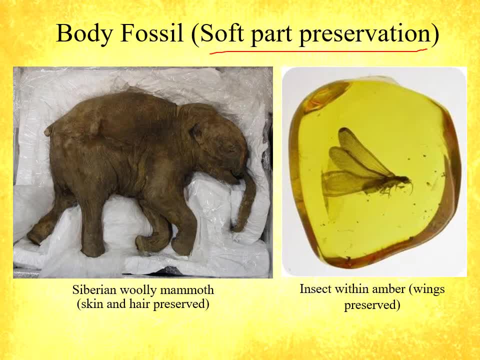 that is completely trapped within the glacier. so as it trapped within the glacier, there, the decomposing bacteria cannot approach to this dead body and due to that, all the soft tissues with the skin of the mammoth and the hair are all preserved. with this uli mammoth. another thing is a amber, that is, the resins from. 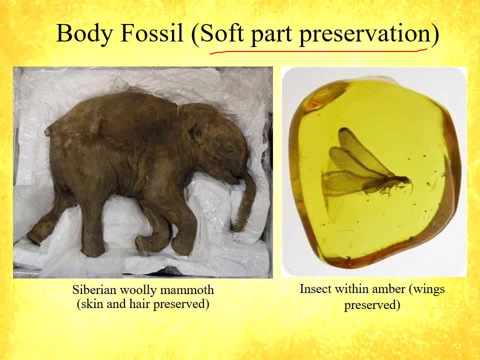 certain plants within this amber, certain kinds of fly or certain kinds of insects are trapped. so it becomes a closed system in which the external affairs cannot affect this dead body now. so the decomposing bacteria cannot get access to act on this insect. so you can see that all the 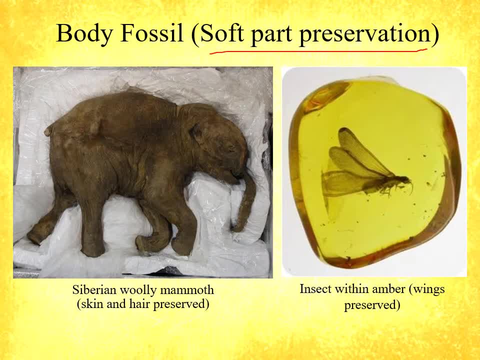 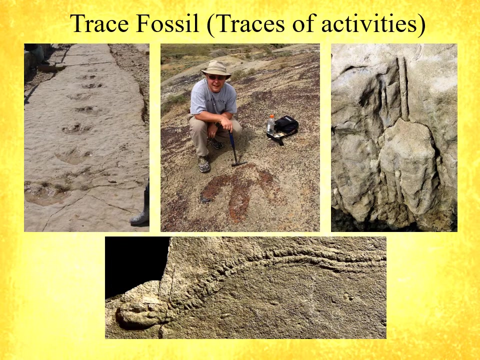 soft body, along with the wings. they are all very well preserved and in just few days ago i somewhere i learned that from these insects the bloods are also collected. this type of insect from a place the bloods are also collected. now these are trace fossils. here the original organisms is not preserved, but their activities. 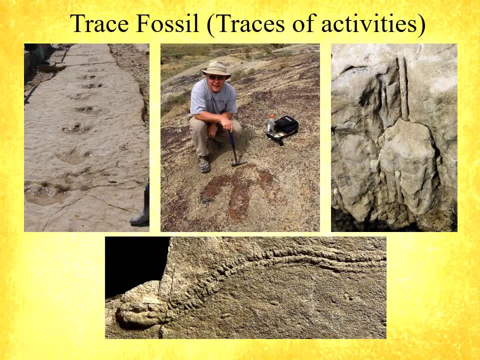 are found preserved in the rock records, such as the dinosaur footprints. you can see that a dinosaur is walking over this sedimentary rock and all the footprints are preserved here. so in the present day, when these human beings are preserved, they are preserved in the rock records. so in the present day, when these human beings 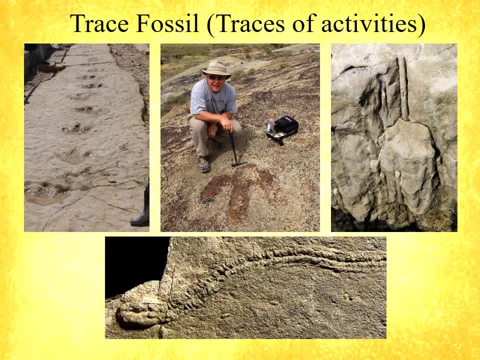 is there. there is no dinosaur, but you can say that during the mesozoic times, instead of human here leaves dinosaurs and they are walking over here and their footprints are preserved in this sedimentary rock. so from this footprint you can get an idea about the size, shape and the ecological 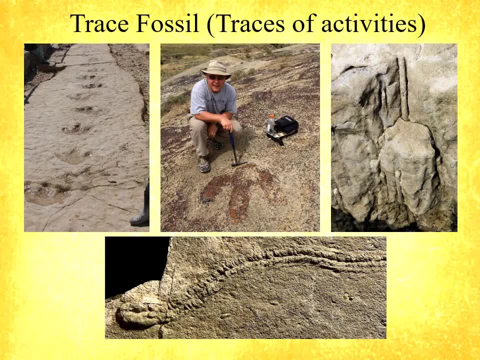 condition and many other things of the dinosaur. Here you can see a burrow. that is a organic body which lives under the subsets. It digs the soft sediments and make a passage to enter deeper part into the sediments and in later stage this passage is filled up by the overlying sediments, So you will get some. 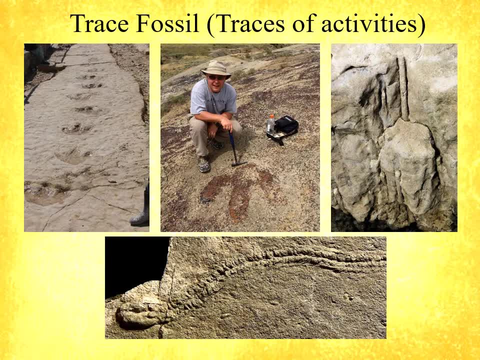 tubular sediment filling. These are called burrows. These are also indicates about the underground habitat condition of any organisms. This is the home of the of any organisms. These are the crawling marks of an arthropod body Organism known as trilobite. They crawl over the surface and during their 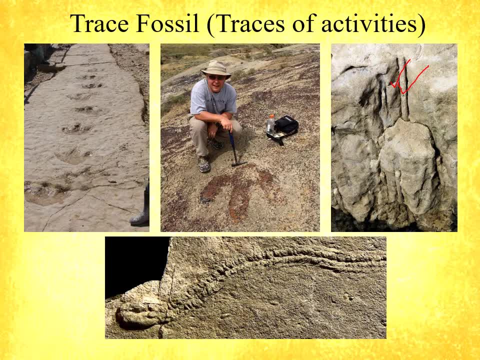 crawling, they make some these kinds of furrows and ridges. So from that you can sometimes say about the size of the organisms, the direction of moving of the organisms, and all these things can be said by the traces of the organic activities, Although the organic body is not found in these cases. 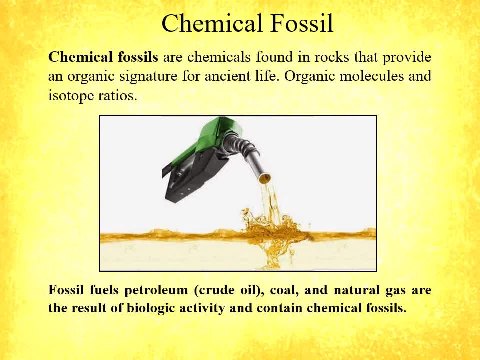 Third, the chemical fossils, where chemicals are found within the rock, which gives indirect signature of ancient life. The chemical evidences are the organic molecules which mixed with the sedimentary rock during the decomposition on some isotope ratios. Whenever an organic body lives in there, it 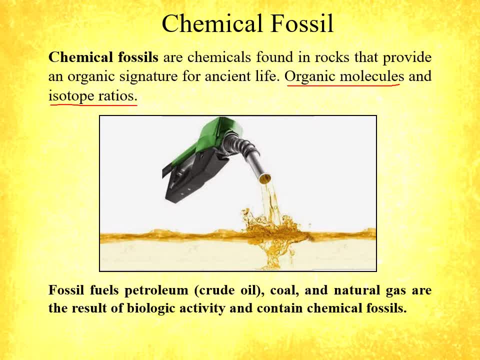 excrete, some excreta which mixes with the sediments and some kinds of isotopes, ratios are changed. So presence of those isotopes or study of those isotope ratio can give you the indirect evidence of certain organisms present during that time. A very good example is the fossil fuels, that is the 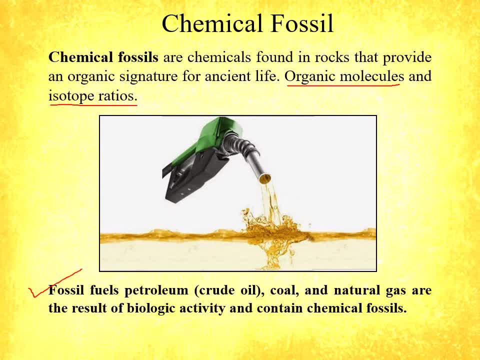 petroleum or coals. The fossil fuels comes from the marine planktons or marine organisms, marine animals, whereas coal comes from the plants. So, although in petroleum or in coal, at many times you will not get the directly the organic body, but instead of that, whenever you get these, 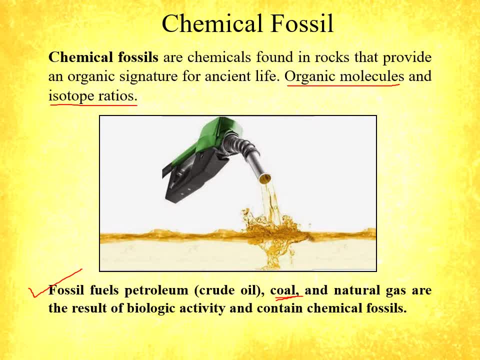 things from the subsurface, from the rock record. you can be pretty much sure that during some time interval, these types of organisms live in these areas and after their death, after their death, they are deposited and with due time they got some modifications, they got some changes into them and 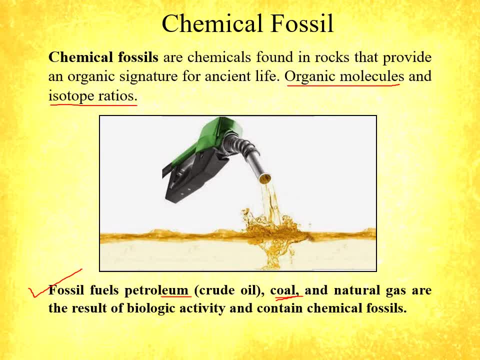 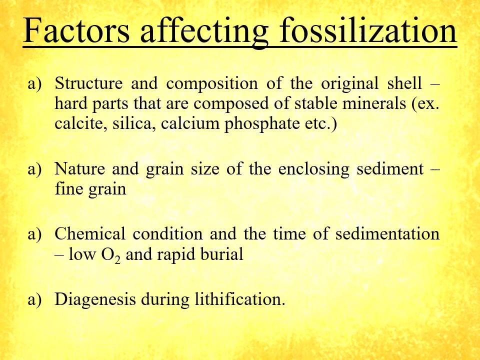 ultimately they form petroleum or ultimately they form coal. So these are the chemical evidences of biological remains, or chemical evidences of biological bodies present during that time. These are known as chemical fossils. Now, factors affecting the fossilization, the structure and composition of the original shell. 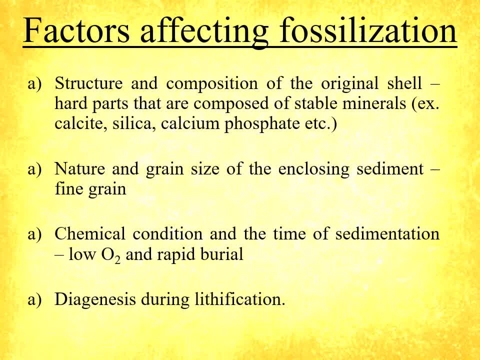 of the hard parts. first of all, i already told you that organism having hard parts and soft parts, the hard parts are more favored. if you compare an organism having hard part and soft parts and another organism having only soft parts, then definitely the organism having hard parts and soft parts. they are favored because due. 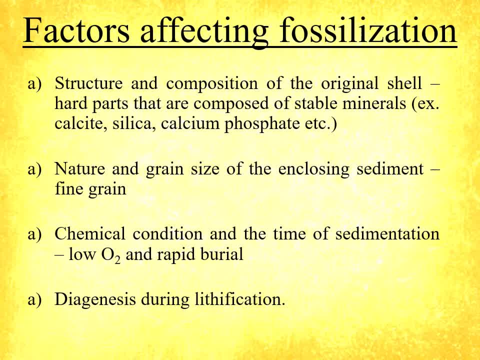 after the death of those two organisms the soft parts are decomposed. so the organisms having both hard parts and soft parts, if their soft parts are decomposed, then also the their hard part remains, so those hard parts can be preserved. but if an organism consists only soft parts, after their 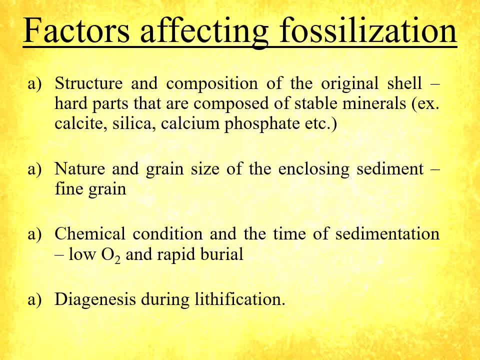 death. if the soft parts decompose then the entire organism is lost from the history. so anything of that particular organism is not preserved. so always hard part bearing organism are favored to be preserved in fossilization. among hard parts, certain kinds of stable minerals are favored in fossilization, such as the calcite, which is a polymorphic. 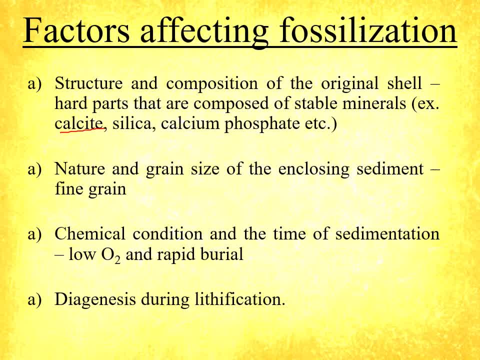 form of calcium carbonate. another polymorphic form is aragonite, but aragonite, for aragonite, is not a stable mineral. rather, calcite is very stable silica, calcium formant. these are the stable minerals. so when an organic body's hard part is made up of these, 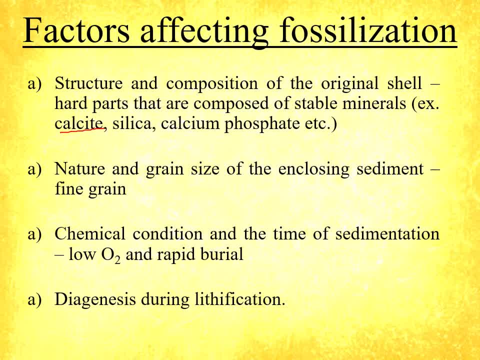 mineral components, they are most readily preserved. second is the nature of green size of the inclusive sediment. so whenever an organism died they have to be deposited with in a sediment basin and they have to be covered up by certain kinds of sediments. now if an organism died in a high energy condition, suppose in the fluvial region in 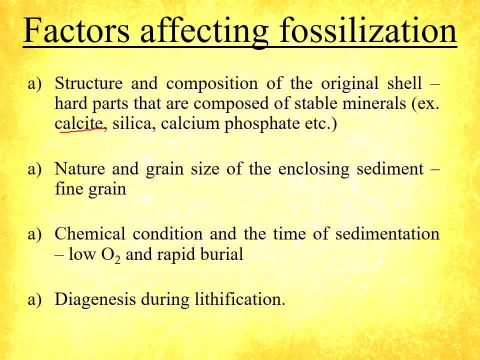 the himalayan tent. so that is the high energy fluvial condition. if an organism died there, so due to this high energy condition, the larger size cluster deposited there and in most cases the organism is destroyed during its transportation. but if an organism dies near the 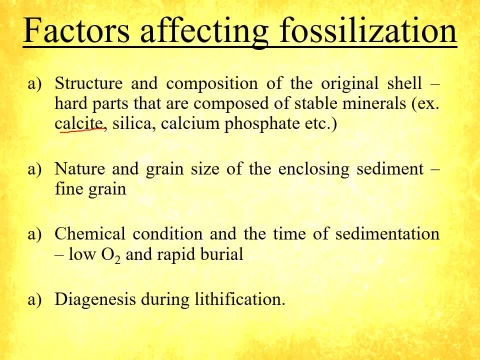 bay of bengal, near the arabian sea, close to the basin. here only the fine grains are deposited. so it's comparably its calm energy condition, a very low energy condition, and here, due to this low energy, after the death of an organism they can be preserved- a chemical condition and the time 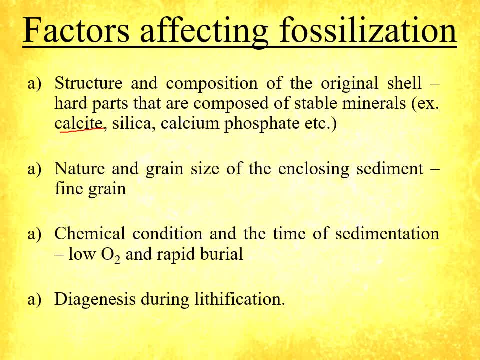 of sedimentation. uh, definitely, after the death of an organism the chemical conditions are not going. required is the low oxygen condition, because in presence of atmospheric free oxygen, the decomposition, decomposing bacteria act readily on the soft mass or soft tissues of the dead body. and when they act on those dead bodies in 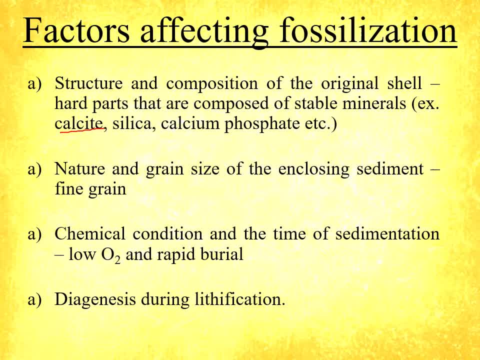 presence of oxygen. they completely destroy the body and no evidence left behind. so if an situation arise when there is low oxygen or there is devoid of atmospheric free oxygen and then the chance of preservation of that organic body is highly favored. so how this low oxygen conditions can be reached? the 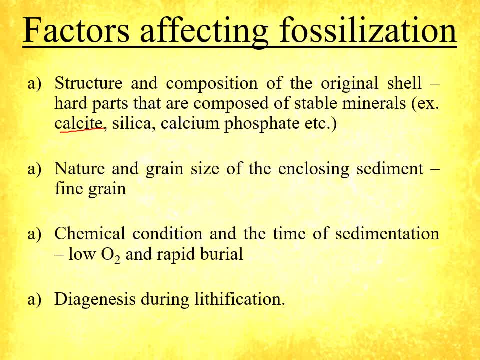 far the very easy way to reach the low energy condition is rapid burial. that means low oxygen conditions can be reached. the very easy way to reach the low energy condition is rapid burial. that means immediately after the death of the organism it will be buried under the sediments. so definitely if rapid burial, quick burial of the dead body by 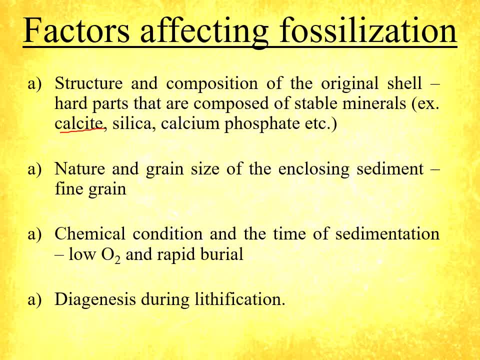 sediments occur then surrounding the dead body. it is completely covered by the sediment, so less amount of free oxygen was there, so chance of getting decomposed becomes very less. so rapid burial definitely indicates that the sedimentation rate in that area must be very high. whenever in a basin, in a depositional set up, the condition 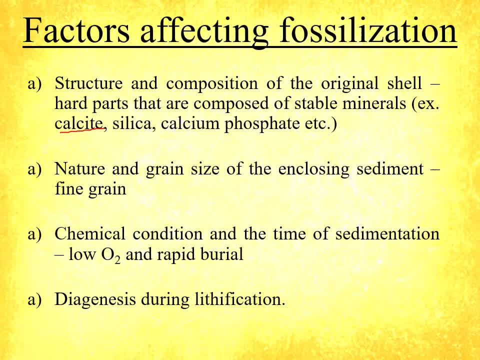 suffers high sedimentation rate and the chance of preservation of the dead bodies of the organisms of those areas becomes very high in comparison a basin where the sedimentation rate is very low. then after the death of the organism, the organism remain exposed for a prolonged time in present in free. 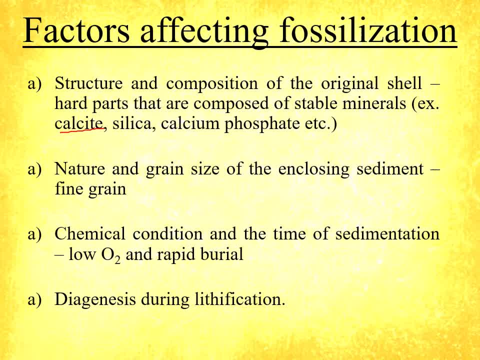 oxygen condition. so during that time the decomposing bacteria acted over it and they destroy the organic body. now this free oxygen does not means that it is the only atmospheric oxygen. free oxygen can present in atmosphere as well as in water. so it does not mean that the organisms after their death deposited underwater. condition that 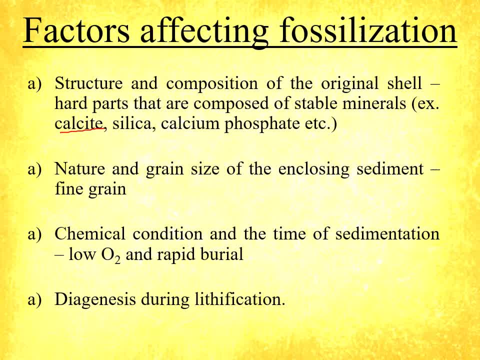 means it will not in presence of free oxygen. in underwater also there are free oxygen molecules. so organism, those decomposing bacteria, can act in open atmosphere as well as underwater in the same way. so for creating a low-energy condition, the first and foremost condition is the basins should have rapid burial. that means high. 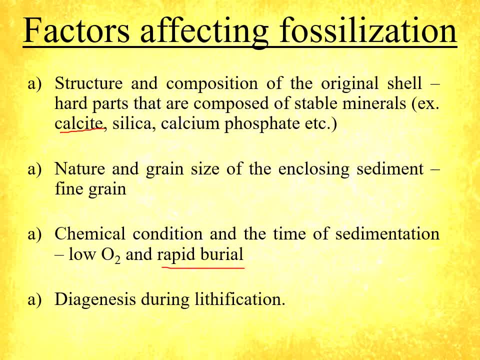 sedimentation rate. and the last one is the diagenesis during lithification. that means all the changes occurred after the deposition of the sediments. those are known as diagenesis. that is, after the deposition of the sediments they are going to solidify and form some kinds of 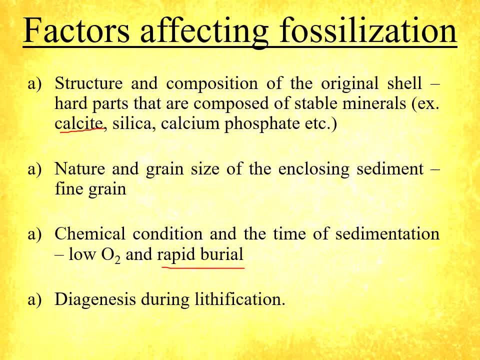 sedimentary rock and during this solidification or lithification of sedimentary rocks, they are suffering certain kinds of changes and these are known as diagenesis. so this diagnosis also affects the preservation of sedum, of the fossils of the ancient living beings. so all these factors that 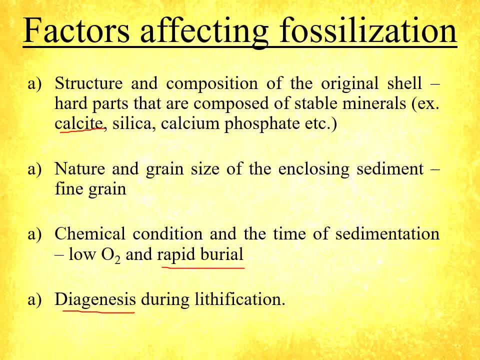 they are play a have a role whether an ancient organisms will be preserved and going to the fossil record or not. if any condition of these things are slightly negative, then in most cases you can have an idea that with slightly negative conditions, you can have an idea that with slightly negative conditions, you can have an idea that with slightly 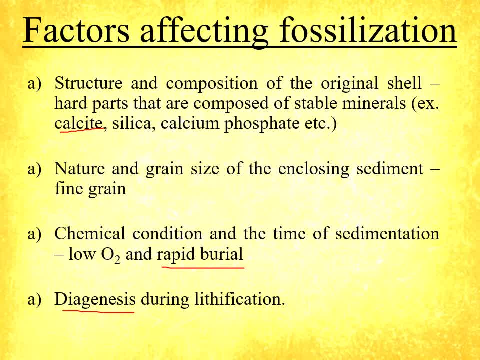 change of any condition. it is most commonly that the organic world, organic change of any condition, it is most commonly that the organic world, organic body, will not be preserved and will not get any evidence of those and living being or will not get any kinds of fossils. so the form, organisms living in 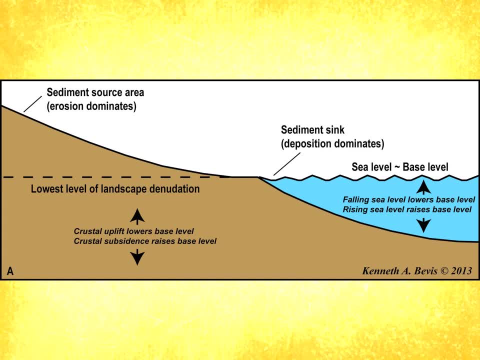 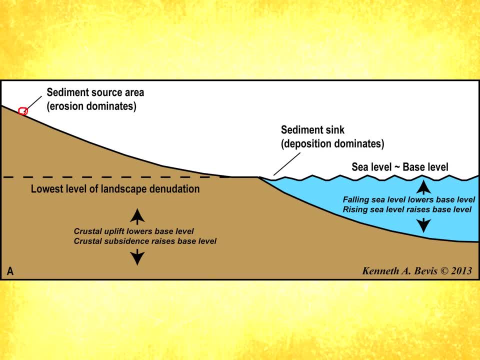 organisms living in the land surface. continental organisms living in the land surface. continental organisms living in the land surface. continental land surface. after they are dead. land surface after they are dead. land surface. after they are dead, they have to be transferred and getting. they have to be transferred and getting. 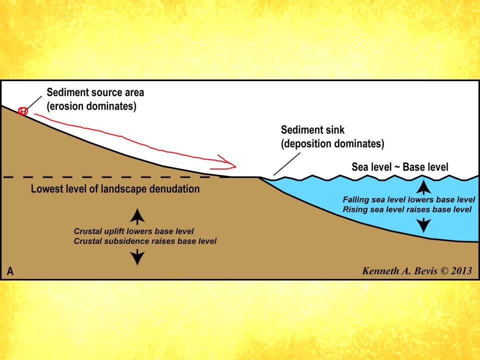 they have to be transferred and getting deposited into the basin. so during this, deposited into the basin. so during this, deposited into the basin. so during this transportation time they are exposed to transportation time. they are exposed to transportation time. they are exposed to the open free oxygen condition. why they 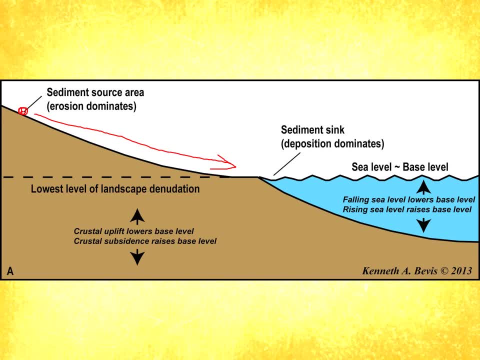 the open free oxygen condition. why they the open free oxygen condition? why they have to transport? because that is the have to transport, because that is the have to transport, because that is the condition, that is the base level of condition, that is the base level of condition, that is the base level of erosion, the mean mean sea level. that is the 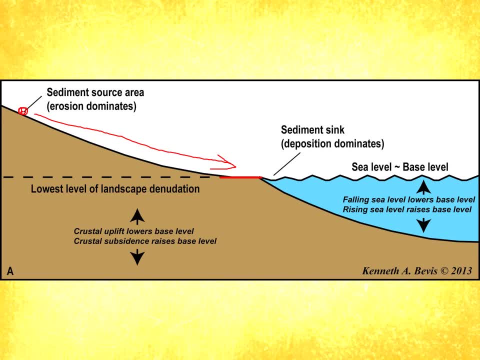 erosion: the mean mean sea level. that is the erosion. the mean mean sea level, that is the base level of erosion, below which no base level of erosion, below which no base level of erosion below which no erosion occurred. so an organisms living erosion occurred. so an organisms living. 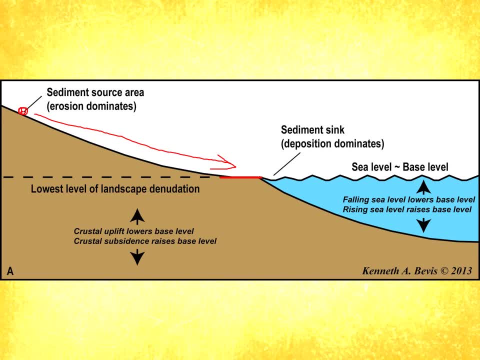 erosion occurred, so an organisms living there after their death, it will be there after their death. it will be there after their death. it will be deposited here. but that deposition is not deposited here. but that deposition is not deposited here, but that deposition is not permanent in sufficient energy. 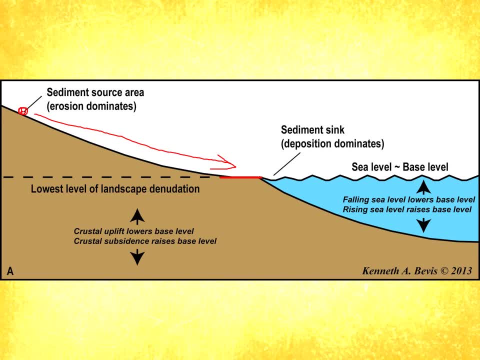 permanent in sufficient energy. permanent in sufficient energy condition: the organisms dead body move condition: the organisms dead body move condition: the organisms dead body move towards the downslope region. only it towards the downslope region, only it towards the downslope region, only it will not suffer any further erosion when. 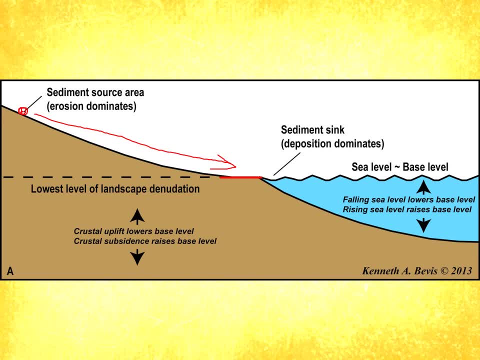 will not suffer any further erosion. when will not suffer any further erosion when. it is deposited below the base level of. it is deposited below the base level of. it is deposited below the base level of erosion, so below the base level of erosion, so below the base level of. 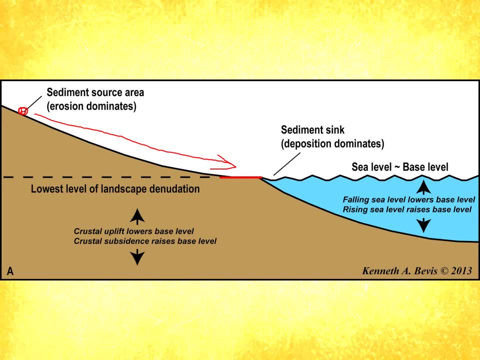 erosion. so below the base level. of erosion that is, below the mean sea level. erosion that is below the mean sea level. erosion that is below the mean sea level: there will be no erosion. so the any. there will be no erosion. so the any. there will be no erosion. so the any organisms deposited below bill mean sea. 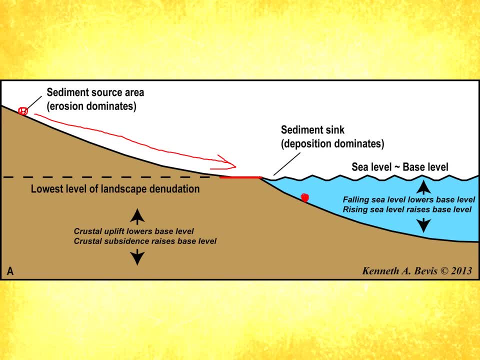 organisms deposited below bill mean sea. organisms deposited below bill mean sea level and their exposure to open free level and their exposure to open free level and their exposure to open free oxygen is very less because they have not oxygen is very less because they have not oxygen is very less because they have not trans. they have not to suffer any kinds. 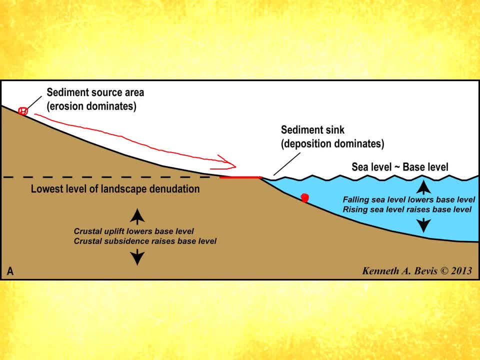 trans. they have not to suffer any kinds trans, they have not to suffer any kinds of transportation. before going to the of transportation, before going to the of transportation, before going to the below the base level of erosion, but below the base level of erosion, but below the base level of erosion, but again, after deposition in the after. 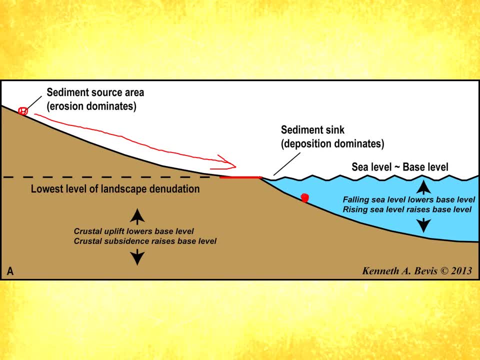 again after deposition in the after, again after deposition in the after deposition: below the base level of deposition: below the base level of deposition, below the base level of erosion: they must be readily covered. erosion- they must be readily covered. erosion, they must be readily covered. that means they have to suffer a rapid 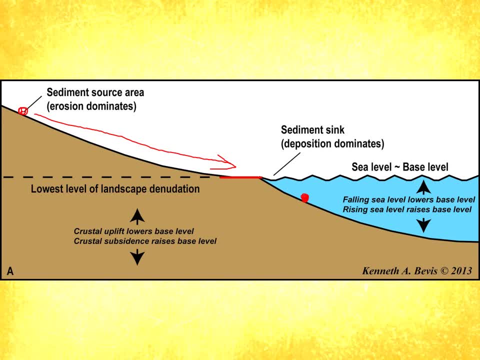 that means they have to suffer a rapid. that means they have to suffer a rapid burial rate, quickly buried by the burial rate, quickly buried by the burial rate, quickly buried by the sediments so that the decomposing sediments, so that the decomposing sediments, so that the decomposing bacteria can affect very, very lesser. 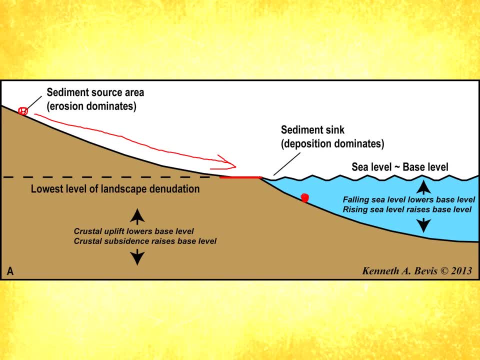 bacteria can affect very, very lesser. bacteria can affect very, very lesser amount to that organic body, amount to that organic body, amount to that organic body. so the organisms living below the base, so the organisms living below the base, so the organisms living below the base level, erosion, they have more chance to. 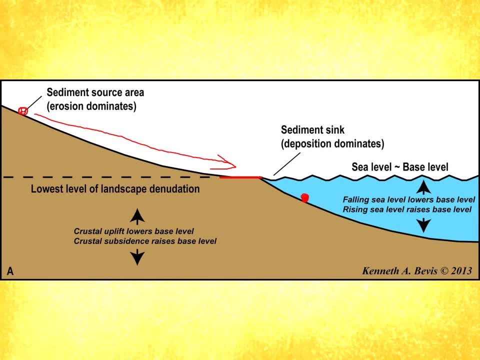 level erosion, they have more chance to level erosion, they have more chance to preservation, whereas organisms living preservation. whereas organisms living preservation. whereas organisms living above base level of erosion- they have above base level of erosion, they have above base level of erosion- they have relatively less chance of preservation. 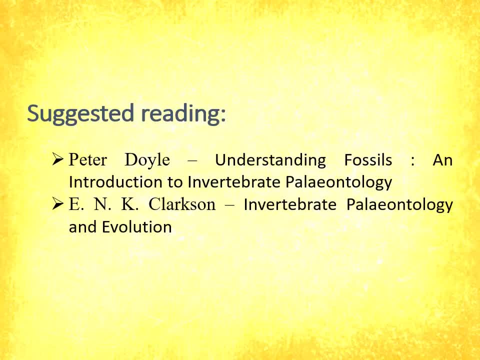 relatively less chance of preservation, relatively less chance of preservation or less chance of fossilization, so or less chance of fossilization, so or less chance of fossilization? so these are the books you have to be, these are the books you have to be, these are the books you have to be followed in this for this class study.